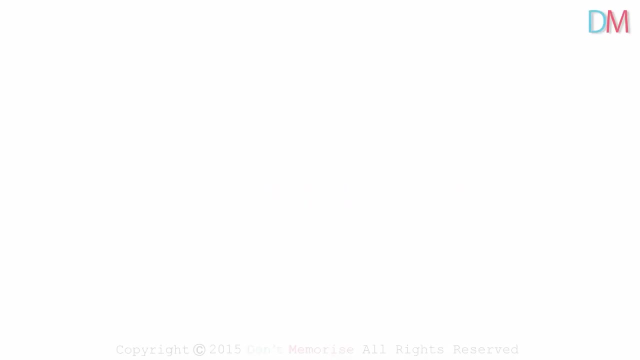 In this video, we will learn something called a symmetric matrix. Yes, a symmetric matrix. When can we say that a matrix is symmetric? Matrix A is symmetric if A transpose is equal to A. Understand this well. The transpose of the matrix is equal to the matrix itself. 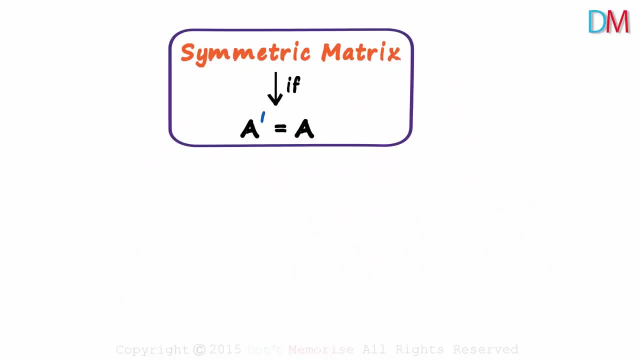 This is the definition of a symmetric matrix. Look at this matrix A. Is it symmetric? What does the definition say? It will be symmetric only if its transpose is equal to itself. So what is A transpose? here We interchange the rows and columns. 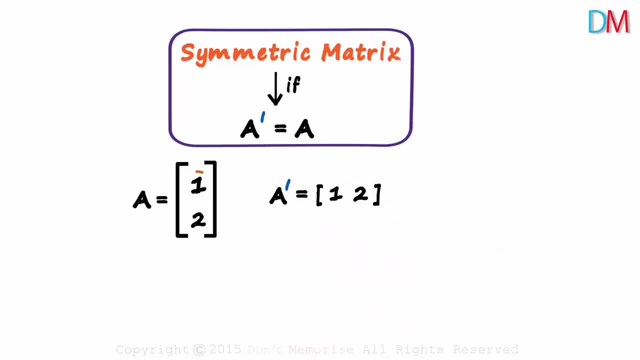 We get A transpose as 1, 2.. The first row became the first column and the second row became the second column. Are they equal? When are two matrices equal? Do you remember equality of matrix? Two matrices are equal if they are of the same order and if their corresponding elements. 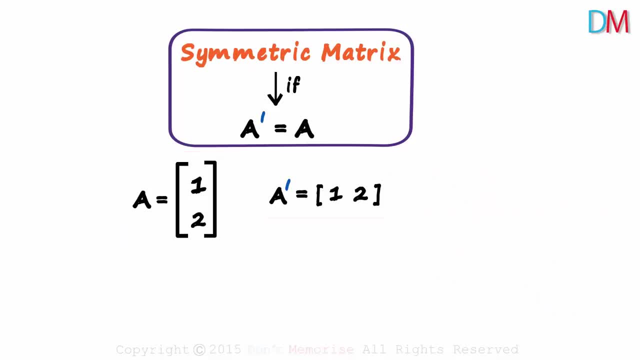 are equal. Here the orders are different. The order of A is 2 by 1 and that of A transpose is 1 by 2.. They are not equal. Because A transpose is not equal to A, we say that A is not a symmetric matrix. 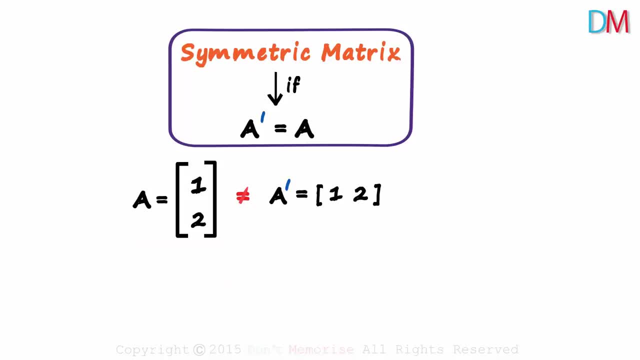 That's how easy it is to find out if a matrix is symmetric or not. We find its transpose and check if it's equal to the original matrix. If not, then the matrix is not symmetric. Let's take another example. Here's matrix B. Is matrix B symmetric? 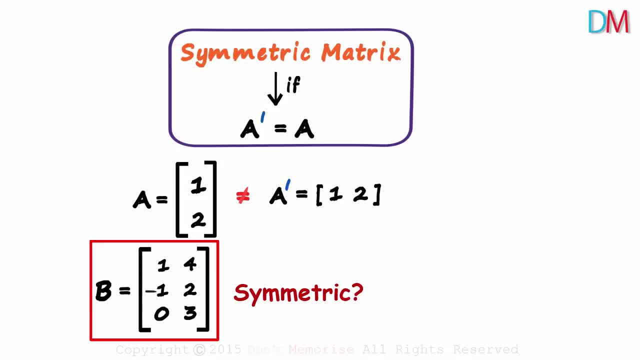 Pause the video and find out if B is a symmetric matrix. To know if B is symmetric, we find B. transpose first: The first row becomes the first column. The first row becomes the first column 1, 4.. The second row becomes the second column. 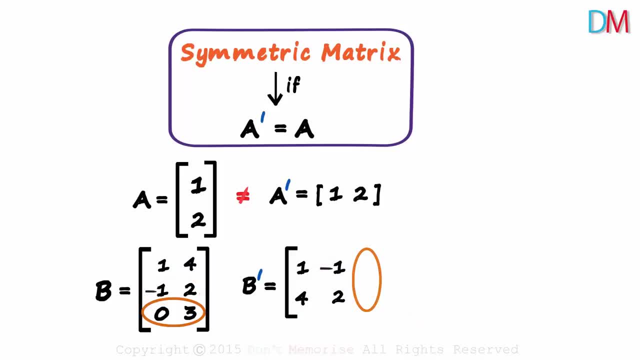 Minus 1, 2.. And the third row becomes the third column, 0, 3.. This is B transpose. Are B and B transpose equal? The order of B is 3 by 2 and that of B transpose is 2 by 3.. 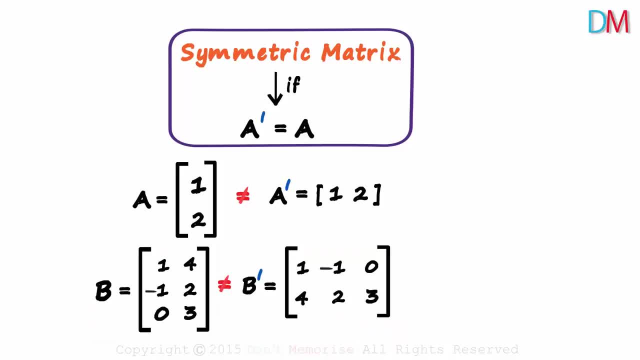 As the orders are different, they are not equal, Which means B is not a symmetric matrix. This should give us a hint. Can a rectangular matrix ever be symmetric? A rectangular matrix is a matrix in which the number of rows is not equal to the number. 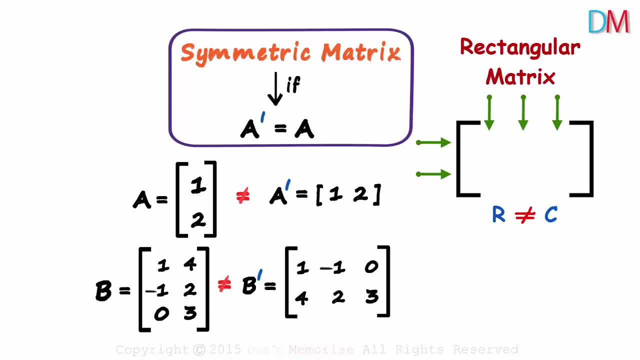 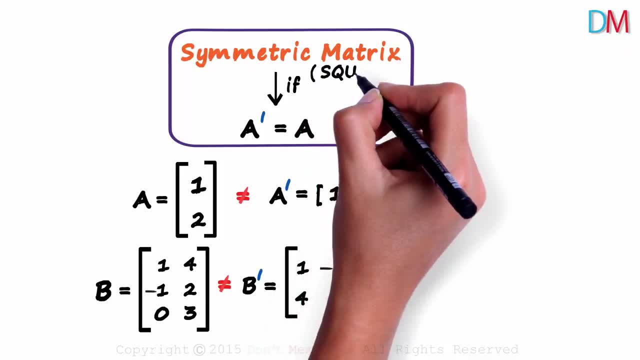 of columns. Can it ever be symmetric? No chance, Because the order of the transpose will definitely be different from that of the matrix. Only a square matrix can be symmetric. A square matrix is a matrix in which the number of rows is equal to the number of columns. 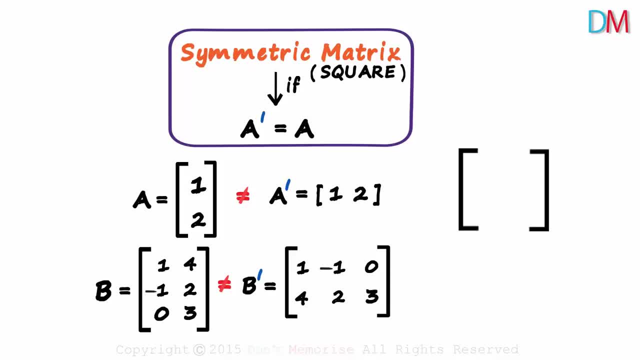 The order of number of rows means that number of columns is simple. Because symbolical matrix is simple, we cannot say that the number goes to any got particular line of colors. We happen to know that equal to the number of columns. Take matrix C, for instance. 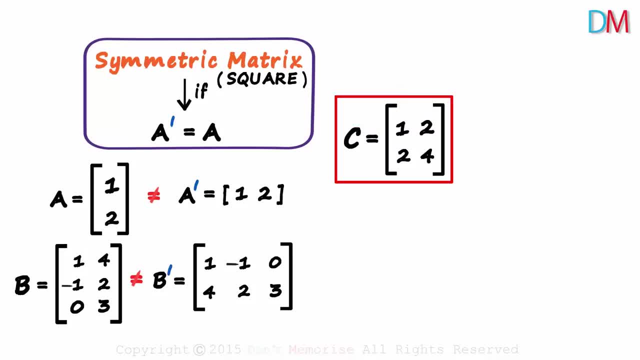 Two rows and two columns. This is a square matrix because its number of rows is equal to its number of columns. Is this a symmetric matrix? We find C transpose to know the answer. The first row becomes the first column, one, two. 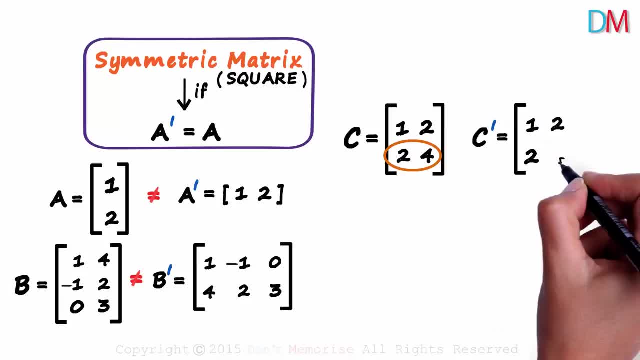 And the second row becomes the second column: two, four. Clearly, the two matrices are equal, Same order- and the corresponding elements are equal: One and one, two and two, two and two, four and four. Matrix C is a symmetric matrix as its transpose is equal to itself. 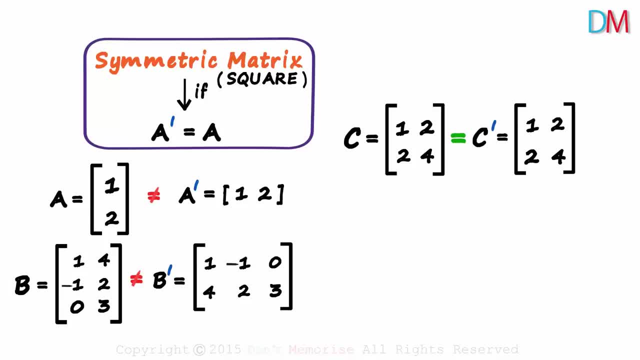 Does this mean that every square matrix will be symmetric? Here's matrix D. It's a square matrix because its number of rows is equal to its number of columns. Pause the video and find out if matrix D is a symmetric matrix. To know if D is symmetric, we need to find D, transpose first. 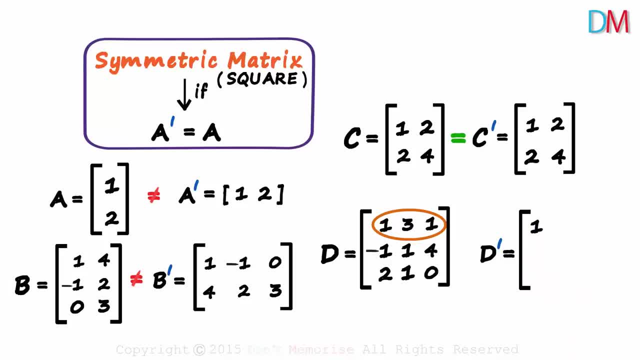 The first row will be the first column here: One, three, one. The second row becomes the second column Minus one, one, four. And the third row will be the third column here: Two, three, one. Two, three, one, zero. 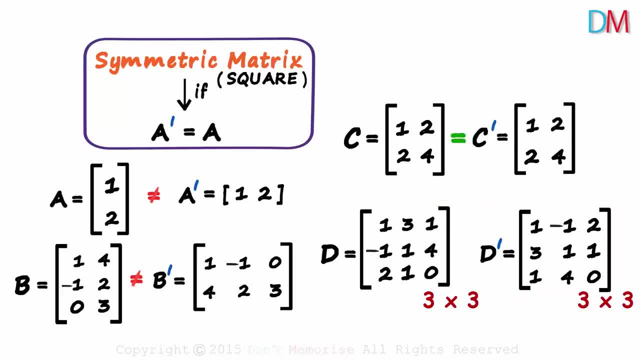 Are these two matrices equal? The orders are equal, yes, But are the corresponding elements equal? Let's check. One is equal to one, Three is not equal to minus one. For two matrices to be equal, all the corresponding elements must be equal.